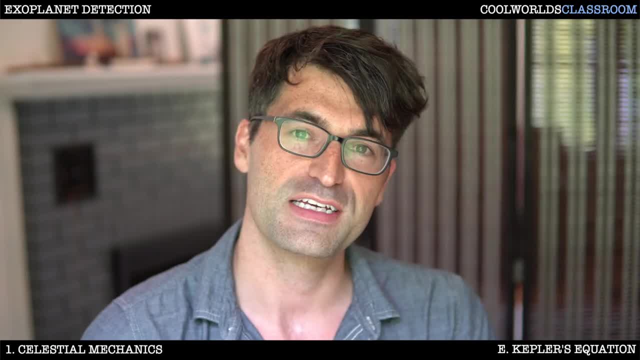 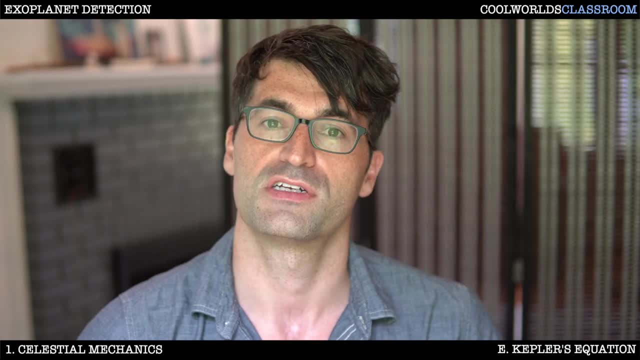 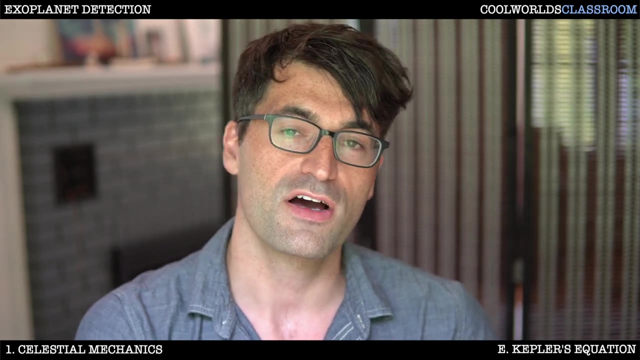 results which we are going to be deriving today. The first is going to be how f changes with time, so that's df dt. The second is going to be how radial position changes with time, so dr dt, or in other words velocity, and then, finally, we're going to be going from time to f. 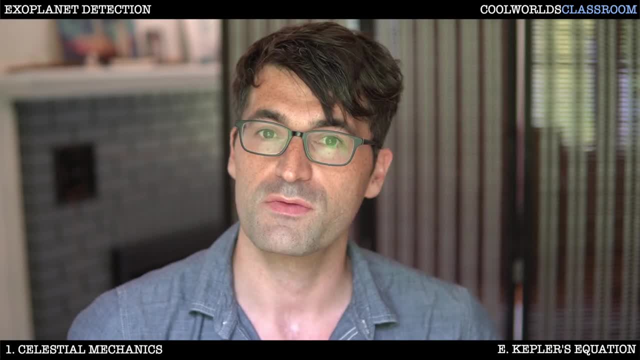 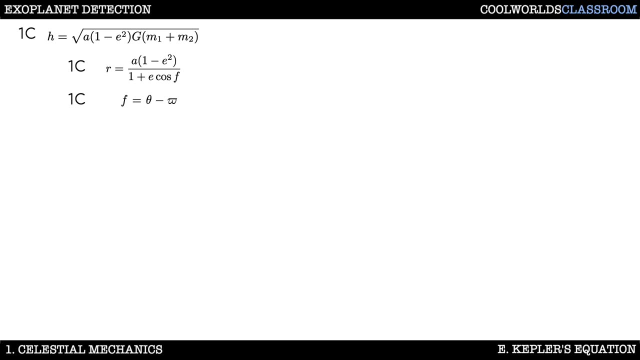 Thinking about a procedure to make that change. we'll start, though, with df, dt. Let's start with the three equations we obtained in video c. These are the specific angular momentum h, the radial distance r and the true anomaly f. We also know from Kepler's second law that h 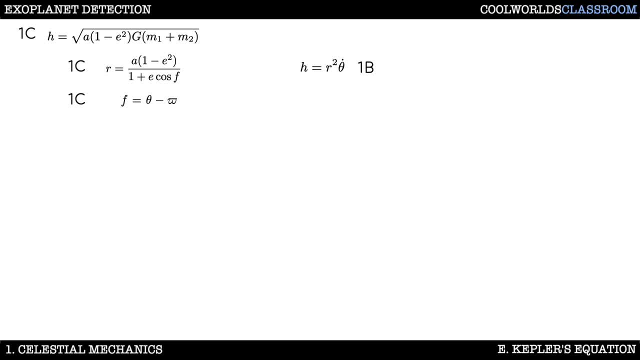 equals r squared multiplied by theta dot, which we covered in video b. Plugging the three equations on the left into the right, we obtain the following: Now notice how, since curly pi is a constant, then theta dot is equal to f dot. Now let's move the a and the one minus e squared terms around a little. 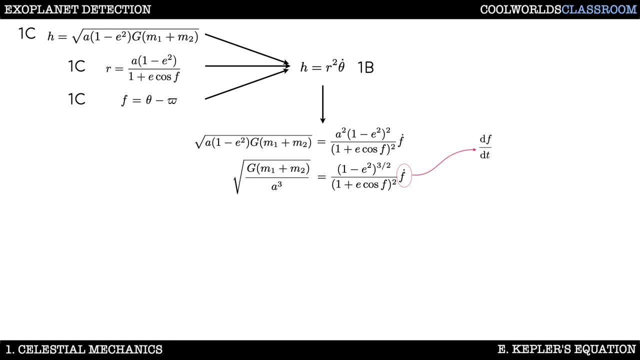 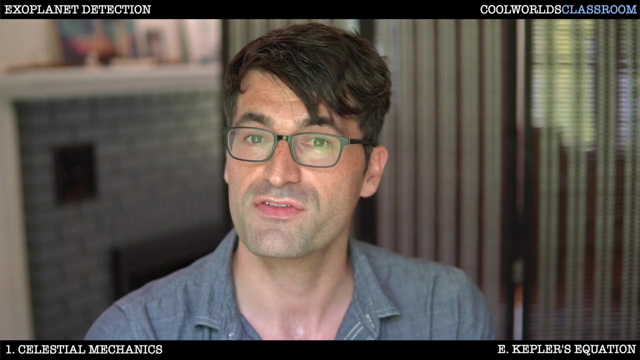 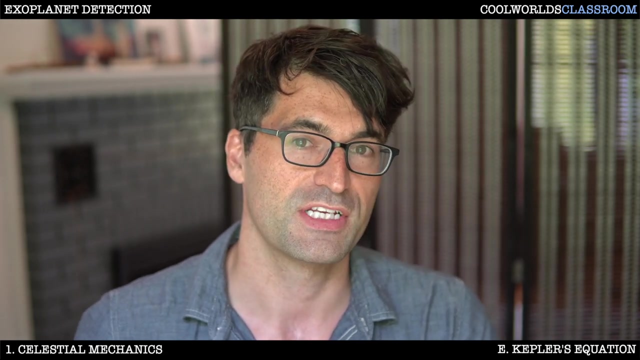 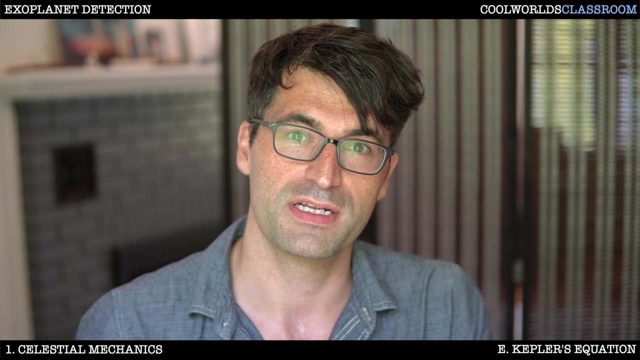 bit. and now, since f dot is df dt, then rearranging this, we obtain dt df as follows: We can clean this up a little bit more using Kepler's third law and replacing this with the third law. Now let's look at this orange term here. Doing so yields the following final equation: Now, unfortunately we can't take this analytic equation for df dt and trivially solve it to get f as a function of time, but we will show a procedure for doing that later in the video. Now, df dt: you can kind of think of it as being like an angular speed, and angular speed is useful. but it's actually more intuitive, maybe more physically useful, to think about the actual function of f. 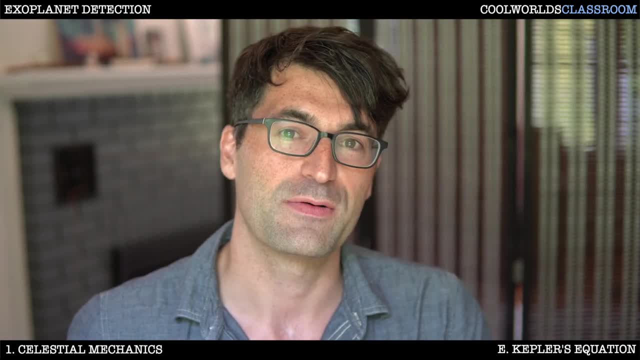 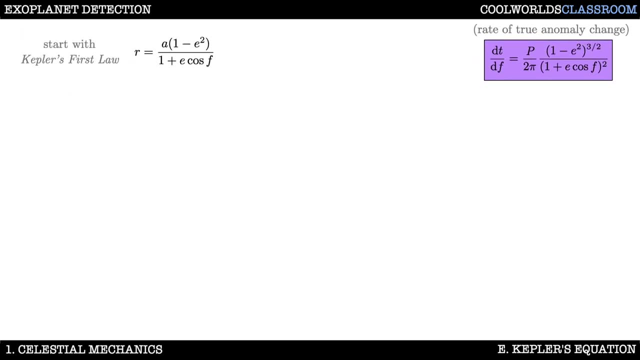 speed, dr dt. So let's turn to that now. Let's clear the slate and keep just these two expressions, Kepler's first law and dt df, Before we can obtain velocity v. we're going to grab an intermediate result that will help us out. First, we can differentiate r to get r dot as follows. Notice how we have an f dot there, which we can now replace with our result from the last slide. Now, looking at this, we can see that these terms here 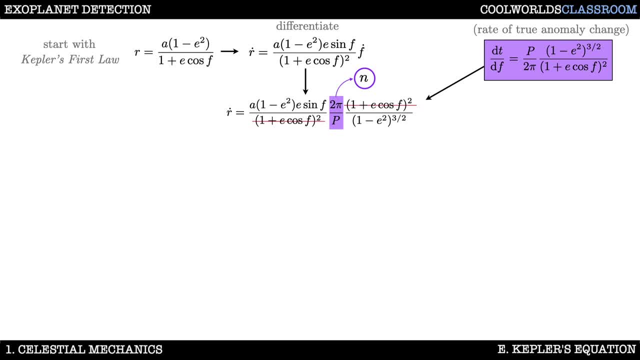 are related to the time it became m or d, Sheriff John magivre. values taken from regular language箔 vs nt. We can also replace 2 pi over p with n, where n is called the mean motion and really just represents the mean angular velocity, which is our total r dot. 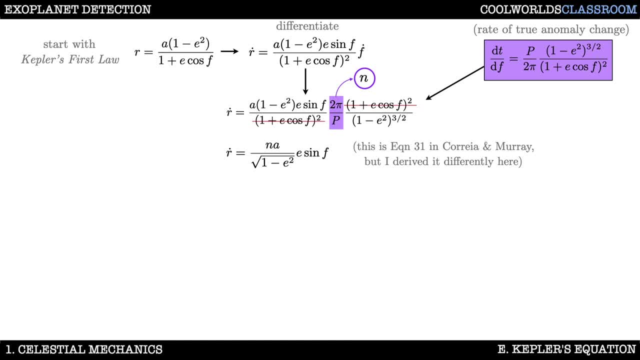 This gives us the following, which is equation 31 in the Correa and Murray chapter, but here we have derived it a little bit differently. Now let's pull that first r dot equation down here. If you look closely, you can hopefully see the r term inside of it, so making that as 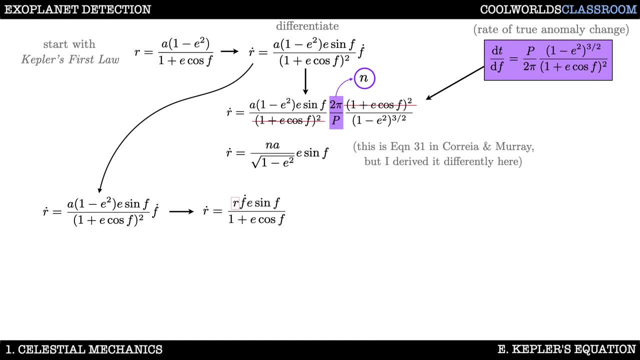 l dot as an integral equal hour. isso sedan is equal to 1r dot in mortality, freed from the inflation. lev, gently, and as itımız��서 replacement gives us the following, where I'm gonna highlight the replaced R with a red box for clarity: We've got R multiplied by F dot together. let's make: 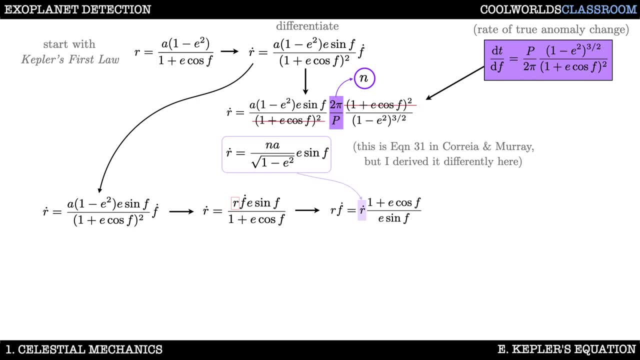 those, the subject as shown here. Next, let's replace the R dot term with a result above it, giving us the following: and here these E sine F terms cancel, so simplifying everything down to just this, and this is the intermediate result that we're going to need Now, before continuing, make sure you can follow. 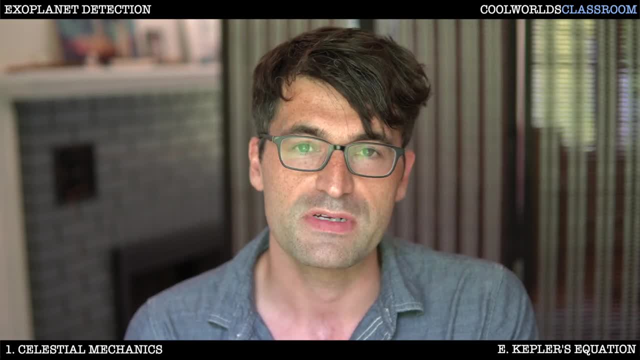 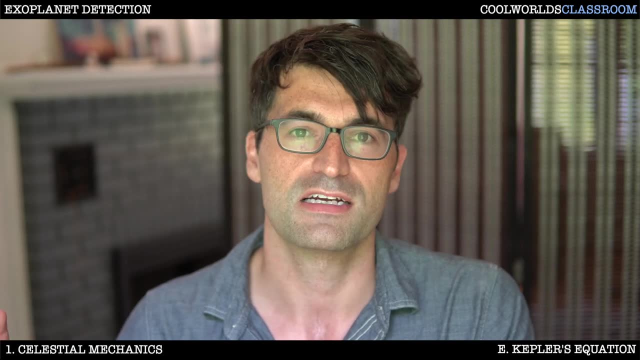 along with all of the mathematical steps there, all of the replacements and the differentiation we did. Now it's not important, or necessarily even particularly useful to memorize these derivations word-for-word. that's not important. but what is important is that you can follow along with everything. 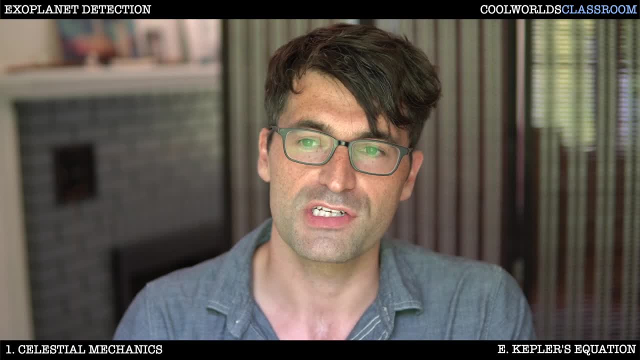 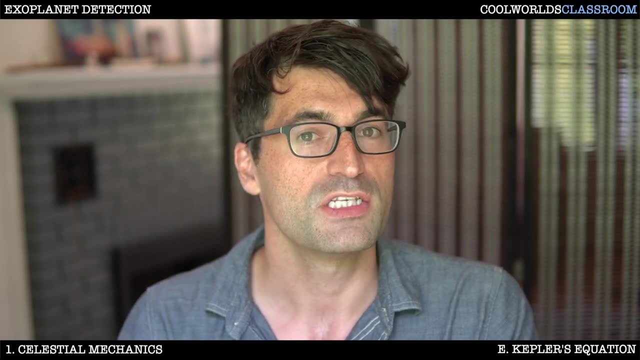 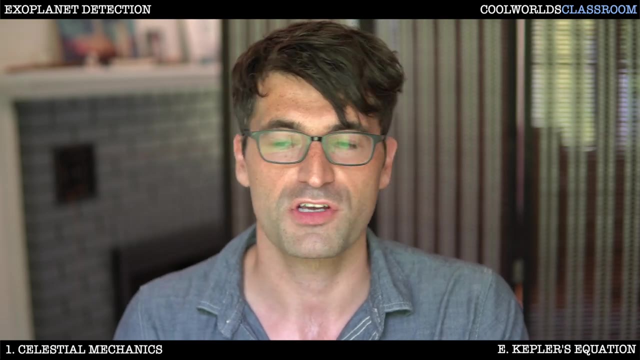 that was done. Why, Well, these manipulations and gaining practice and doing them over and over again? it's like training a muscle you, The more we do it, the more second nature it becomes to us. My goal here, as your teacher in these videos, is not just to show you where these laws come from and 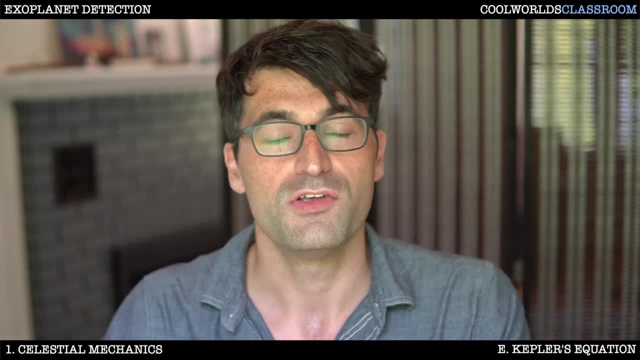 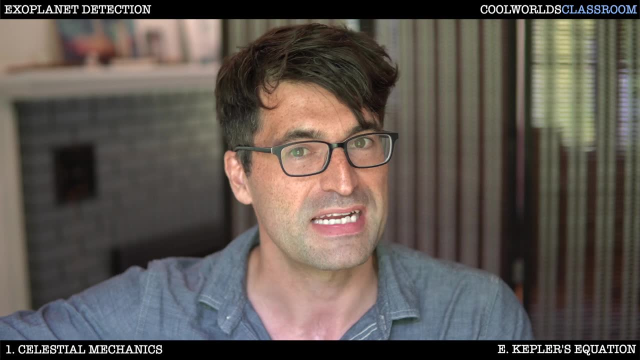 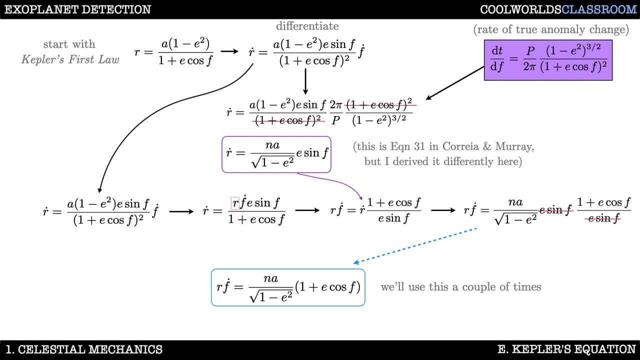 these methods come from, but to equip you that you really could come up with your own new methods in the future to detect exoplanets, exomoons, rings or whatever, using the principles of these manipulations that we've talked about. We're now ready to get velocity. Let's keep these two results and move the. 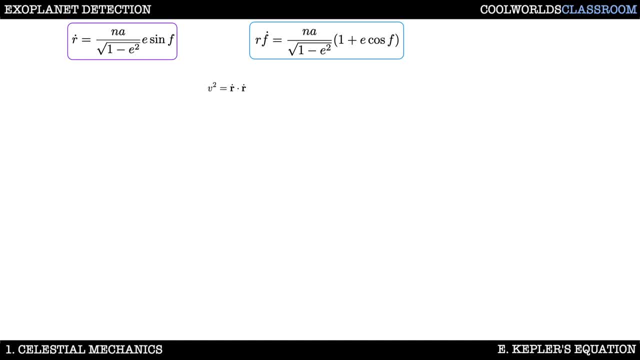 той over to a new slide. We first note that V experienrove i' going to be the self dot product of the r dot vector. Now, recalling our polar coordinate expansion for r dot, we have the following: using this to take the self product, it's just gonna be the square of the two components added. 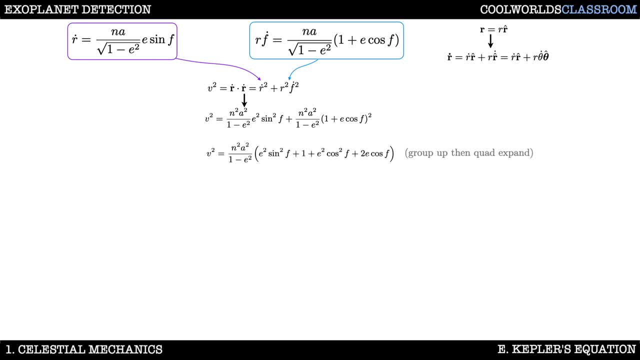 in quadrature. Let's take the common factor out as follows. we now notice a cosine squared and sine squared term that will add to unity. to simplify this, Next, we're gonna add prix-classique. this ok, but we're going to add plus 1 and minus 1 inside the bracket, which of course we're allowed to do, and 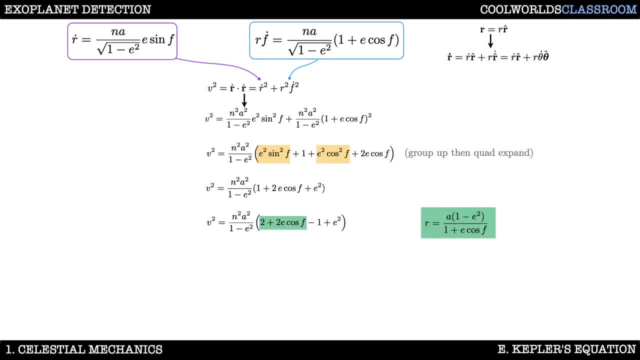 that gives us this and, by comparison to our r equation, we can replace the 1 plus e cosine f term here with r. after doing so, we find a common 1 minus e squared factor that cancels out, giving us the following more simplified form: now this looks like a lot of steps, but i'm really just. 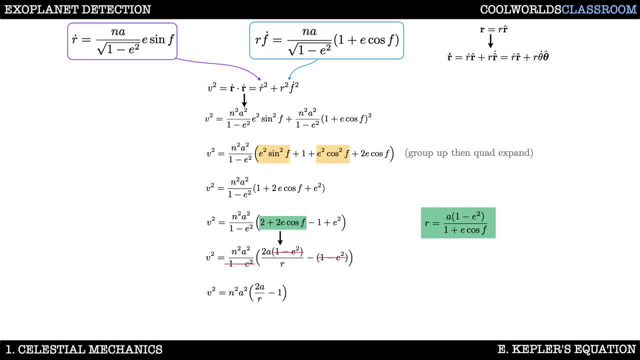 breaking down all of the little steps often skipped over in this derivation. finally, we can replace n squared a cubed using kepler's third law to get our planetary velocity as follows. now, as a test of your understanding, i want you to take this equation and write down an expression. 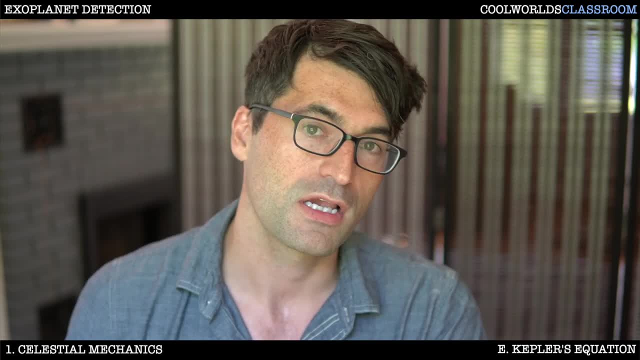 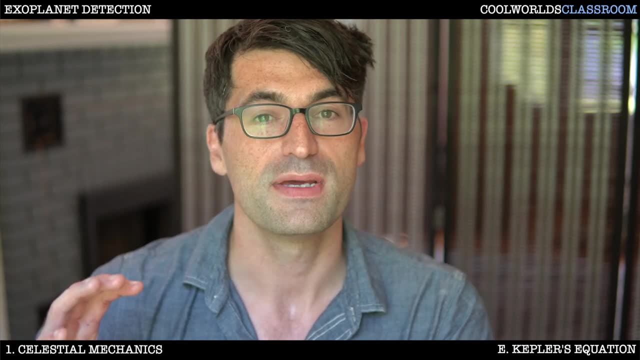 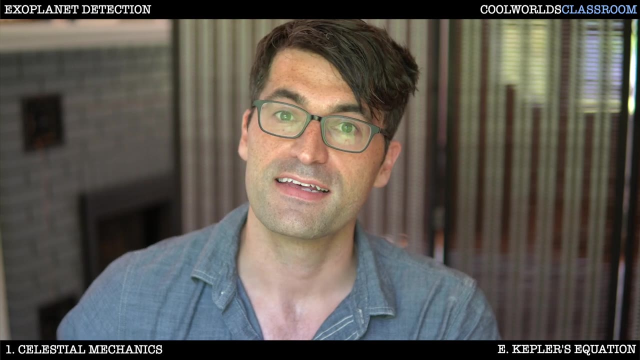 for the velocity of a planet, but in the limit of a circular orbit. so just imagine that e equals zero and solve that equation. now i want you to take that saved formula and compare it to a second, completely independent way of getting the circular orbital velocity instead. this time i want you to 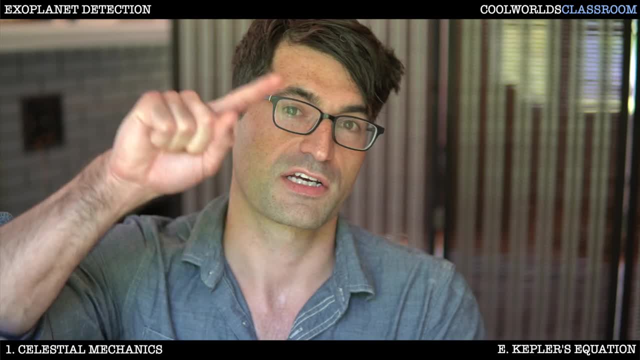 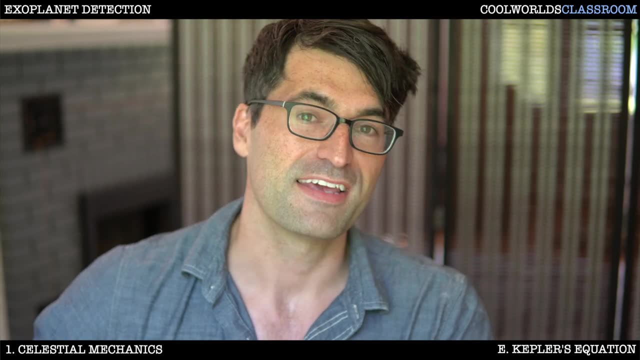 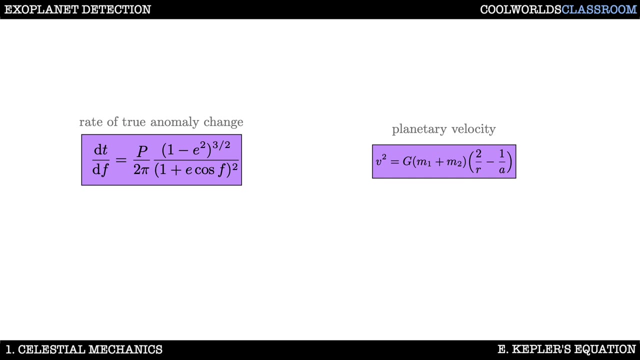 do you? to do this, we need to write r dot in terms of just r, so that we can solve the equation. let's take these, these three results, and move them over to a new slide. now, by simple rearrangement, we can write r dot squared as follows. notice how the terms on the right hand side are things that we have. 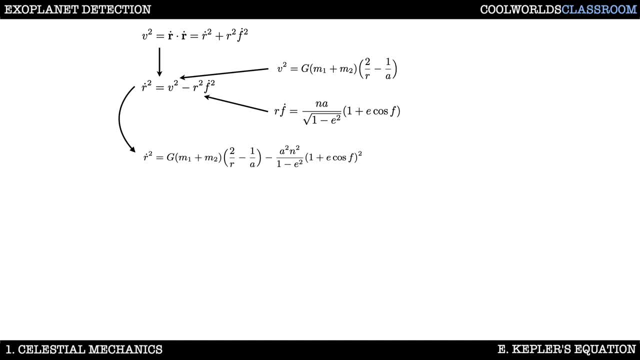 solutions for now. so let's plug them in. remember that what we're trying to do is to write everything in terms of r. so let's now recall kepler's first law to replace the 1 plus e cos f term here. similarly, i'm going to use kepler's third law to switch from the massive 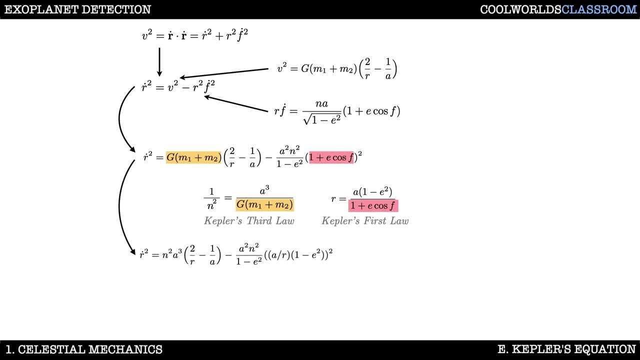 to n squared a cubed. this gives us the following: check you follow along, we can multiply out that bracket on the right to get this and finally, taking a square root and pulling out the common factors, we get what we want: r dot in terms of r, no f's remaining. this is a differential equation. 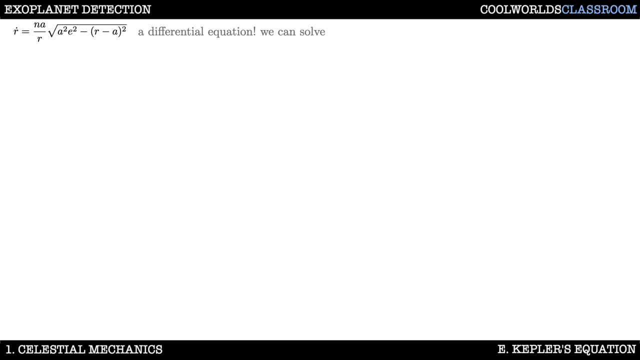 that we can solve. let's bring it over here. the fact that r appears in two places on the right makes this tricky to solve. so to make progress, we'll do what we often do with such equations and make a substitution. let's define a new angle: capital e as the eccentric anomaly, defined as follows, as you can see in the 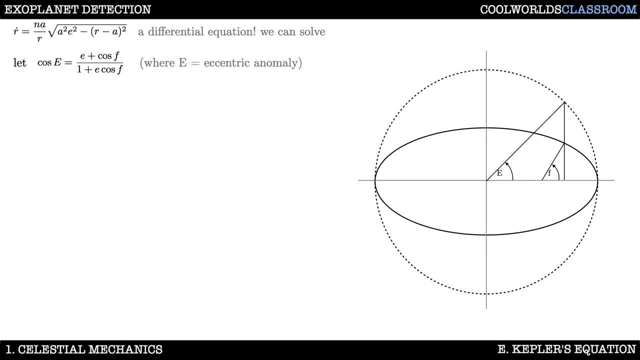 top right. this has a geometrical interpretation by imagining a circle of the same semi-major axis as the orbit, with e subtending an angle from the planet to the circle center. so with that substitution our equation for r becomes this a bit simpler and we can obtain r dot by differentiation. 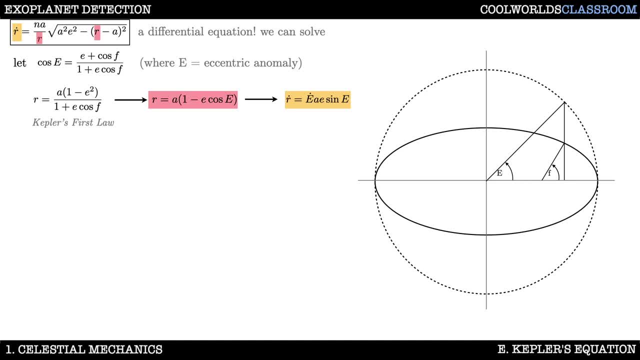 so using these in our differential equation, we get the following- and hopefully you can see that there are going to be some things which cancel out here. after making the cancellations, we get this, but that one minus cosine squared term is really just a sine squared term on the inside. so pulling 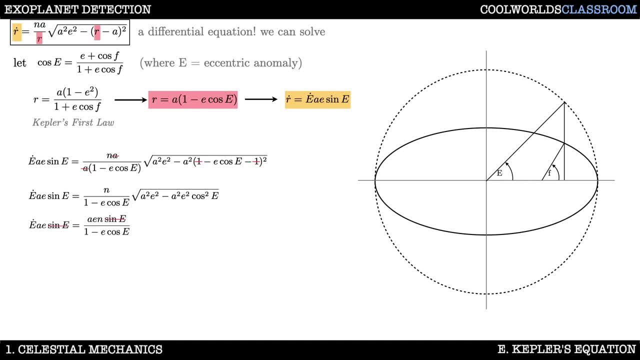 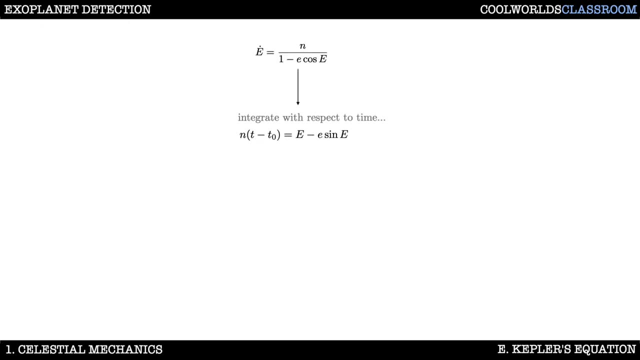 that out. it cancels that with a left-hand sign, and so finally we get this cute little equation in e. now we can actually just directly integrate that to give us the following equation for how e evolves with time, taking the two results over to a new slide. let's look a bit more carefully at 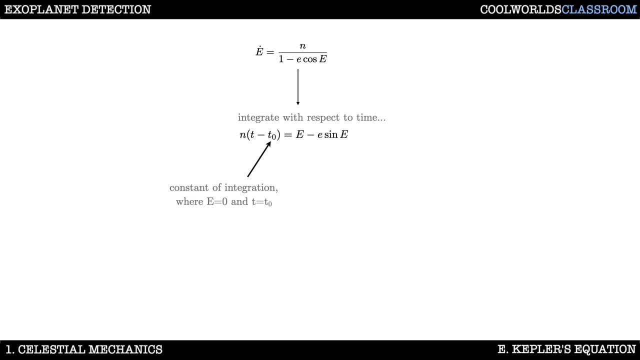 this. the t naught on the left is just a constant of integration. the term on the right hand side, by comparison to the left, is just something which is proportionate to the left side of the equation. so if we take the two results over to a new slide. 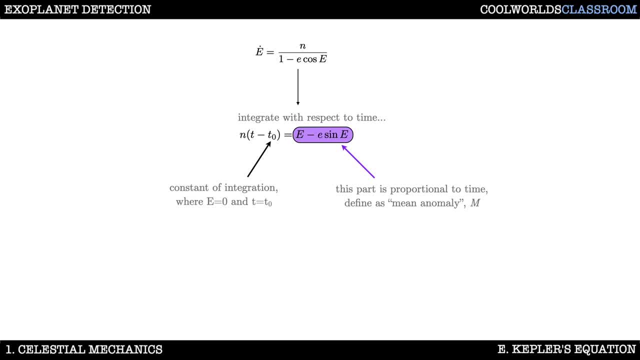 we can see that the t naught on the right side of the equation is proportional to time. let's call that whole thing a new angle. mean anomaly, capital m. that replacement also defines kepler's equation, which relates mean anomaly and eccentric anomaly together. so that means altogether we have three. 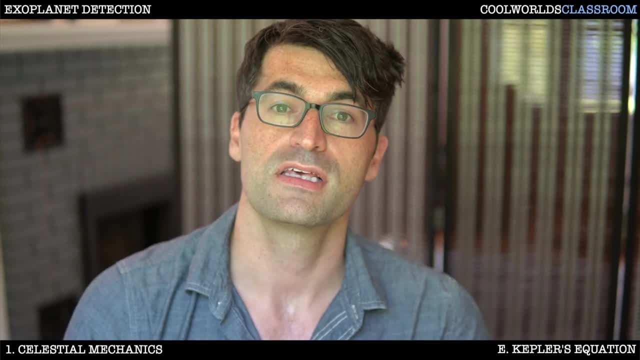 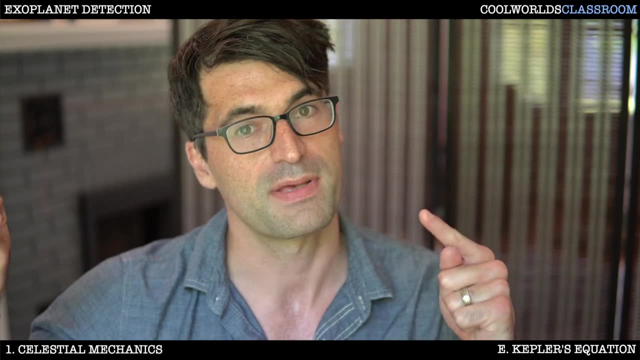 angles describing a planet's position. we have first the true anomaly f, that describes the angle subtended from the planet's position down to the star and back out to the periapsis position. that's f. second, we have the eccentric anomaly, capital e, and that's really just a. 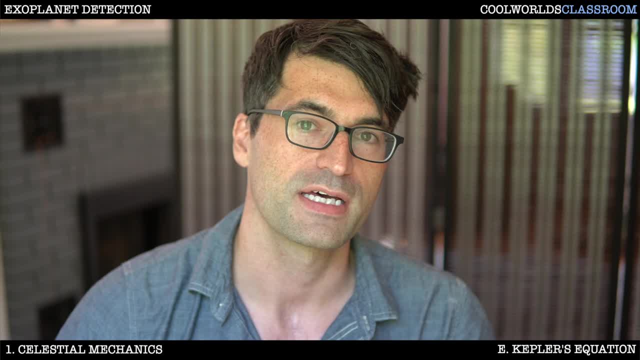 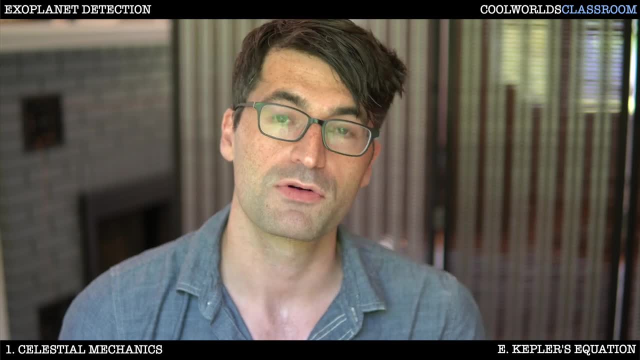 geometrical transformation of f. it's like stretching this orbit out a little bit. and then, third, we have the mean anomaly, angle capital m, and that's really just defined to be linearly proportional to time. and these three angles together form a kind of holy trinity when we're trying to solve for. 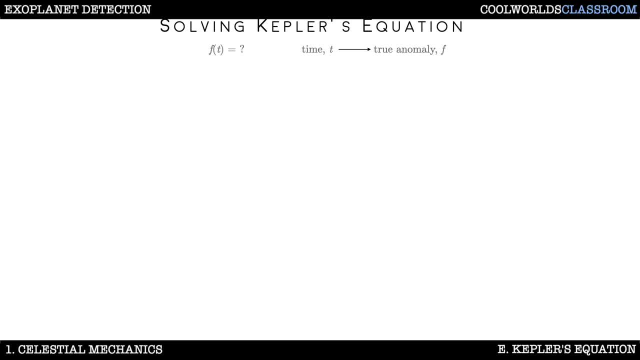 orbital mechanics. finally, we can now present a recipe for turning times into true anomalies. this is extremely valuable when modeling exoplanet orbits, and it sits inside almost all codes and software for detecting exoplanets. so here we go. step one: we define mean anomaly as a simple linear 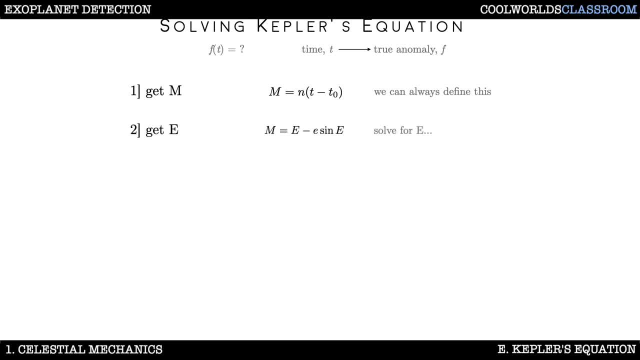 function of time. step two: we relate this mean anomaly to eccentric anomaly in order to solve for capital e. now, unfortunately, this equation is transcendental, which means we can't analytically solve it. a popular numerical approach is to use newton's method. yes, as in isaac newton, that guy really does get around, which, when we expand it out. 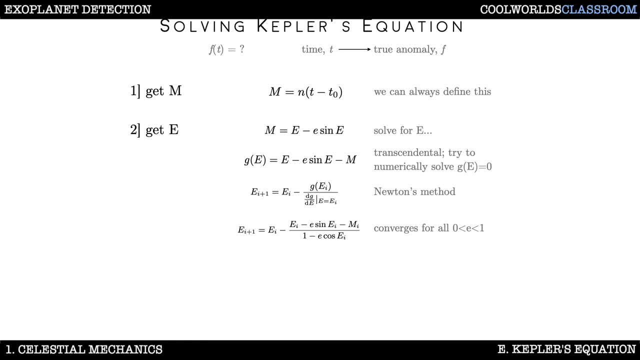 gives the following recursive formula that converges very quickly. now step three: we take these eccentric anomalies and turn them into true anomalies using our geometrical relationship. from before. this is usually done using the following more elegant equivalent expression: now we've run out of time today, but we'll actually go over some real computer code to do this soon. but 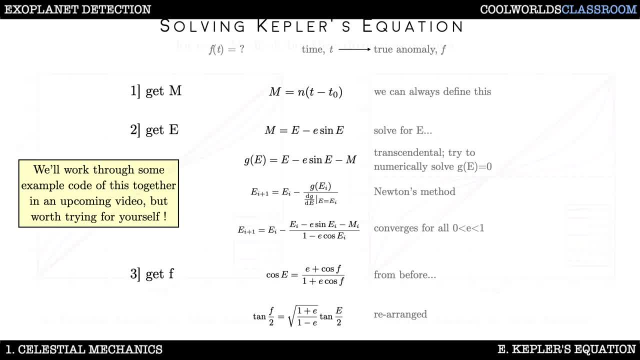 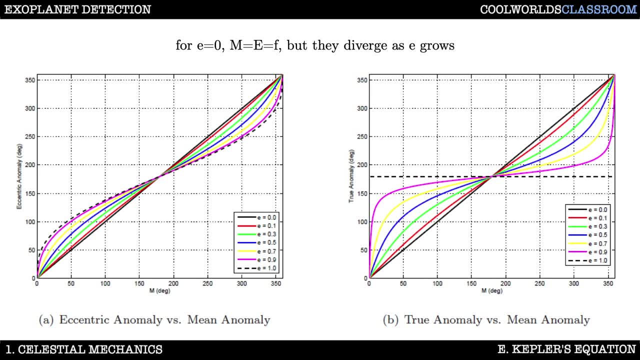 let's start taking a look back at the video привет. it's a different video. in this video, i don't think that every computer can produce a full program. this time we're familiar with the term, which can be used toивive. it's as фотографova aut: instructing you to create a brightness. 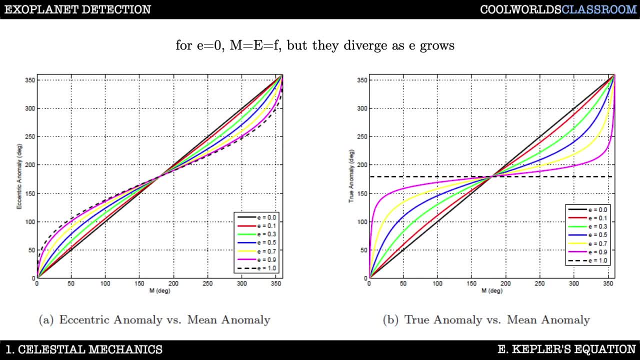 sensor. it takes our to the example. let's say we want to have a fficient line uing i, a 6.9.. We have mean anomaly on the x-axis here which, recall, is a proxy for time. So you'll notice that the planet spends a lot of time at a true anomaly angle close to